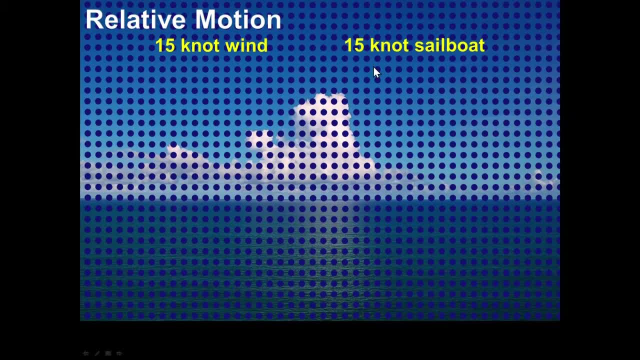 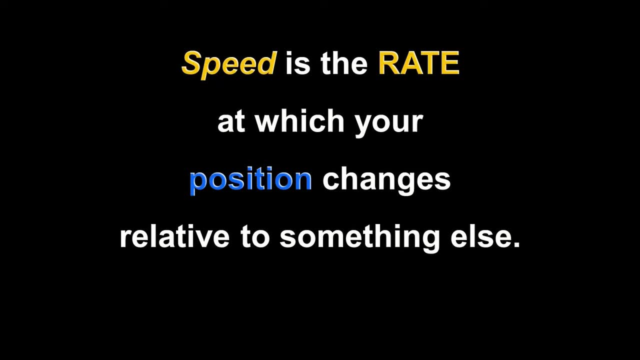 There's not going to be any wind blowing into the sails, So that situation couldn't happen like that. Alright, so now that we know what movement is, or just motion, let's talk about speed. Speed is the rate at which your position changes relative to something else. 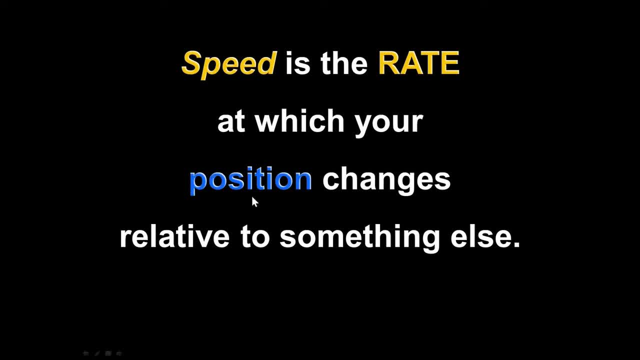 And so if I am in one position, like 5 feet away from the wall, and then I move to another position, say 10 feet away from the wall, and I do that in one second, I can calculate the speed that I changed my position. 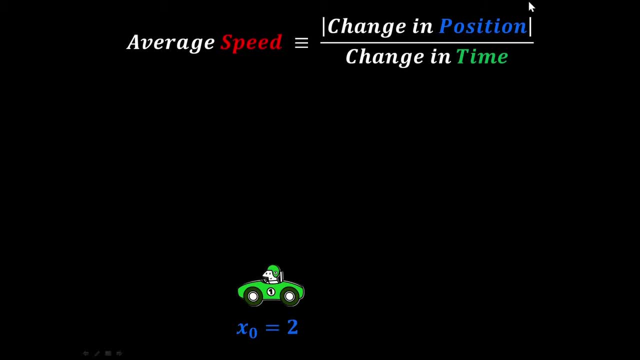 So here's an equation: Your average speed is the absolute value of your change in position divided by the change in time. So, just like we did with change in position, we could start a stopwatch, and at one instant the stopwatch might read 10 seconds. 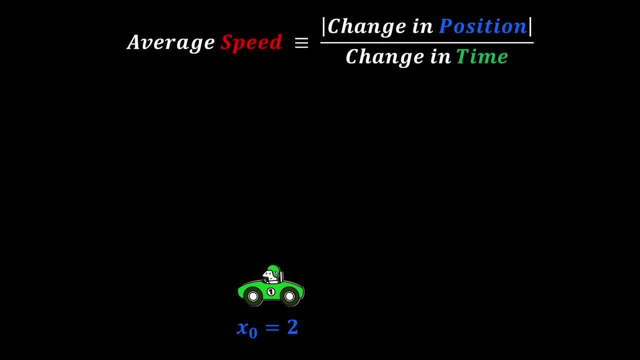 A little while later it might read 20 seconds, So the change in time was from 10 to 20, or just 10 seconds worth of time. So here we are, in its initial position and it's going to move to some final position. 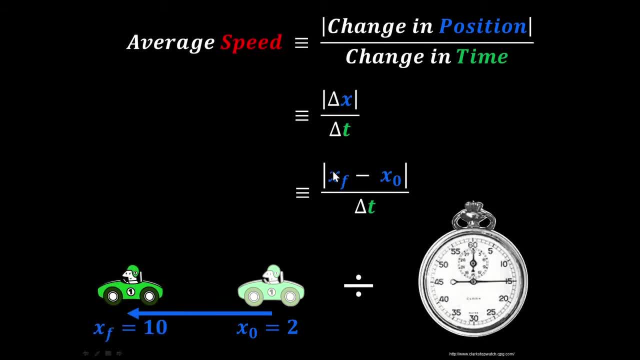 We can calculate the change in position by taking the final position. the final position, your x-coordinate minus your initial position, And this is the letter 0, sorry, the number 0. It is just saying where were you the moment the stopwatch started. 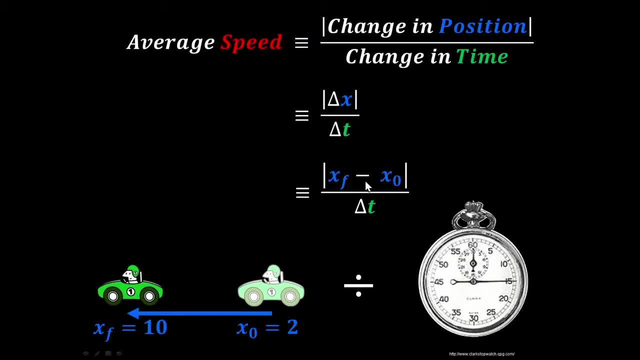 So, at time 0,, what was your position? And what was your position finally? So you just take your change in position and divide it by time, All right. And when you take the change, The change in position, that's just simply the distance you traveled. 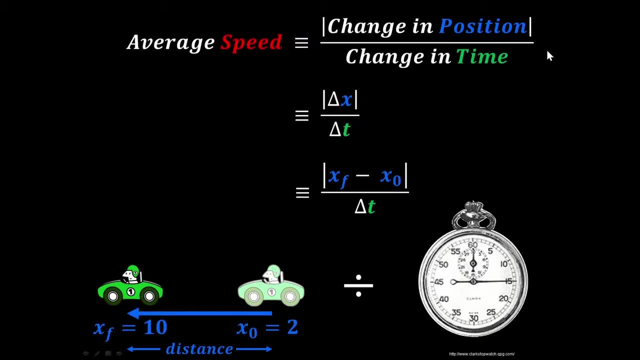 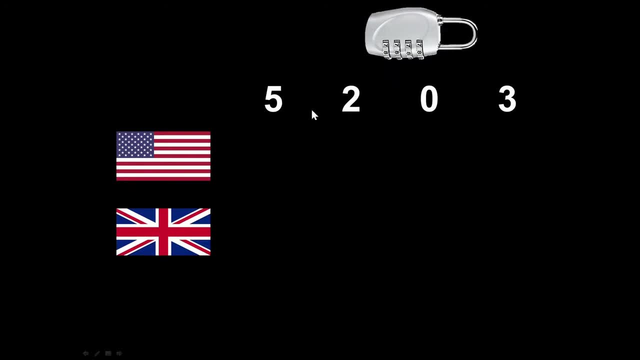 With average speed. it is just the absolute value. We're just looking at the total distance you traveled. Now let me explain a little bit more about that. 0. In America, if someone were to give you the combination to their code, 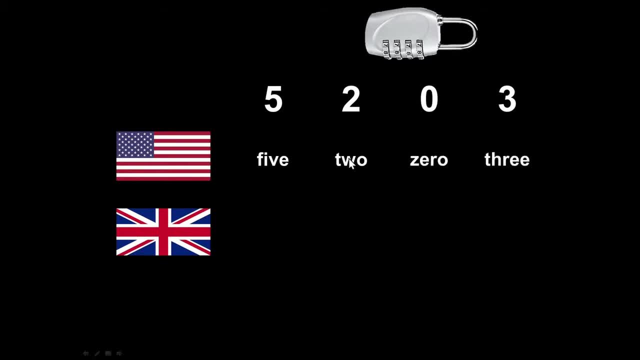 they might say 5,, 2,, 0,, 3.. Across the pond they would probably say 5, 2,, 0,, 3.. And 0 is a word that they use for 0. So when I said, this was the position at time- 0,. 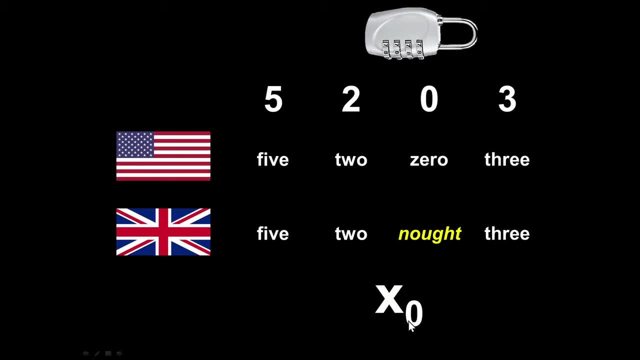 the way we say that is v, It's a subscript. sorry, It's not v, it's x And this is a subscript. So we say x sub 0.. x sub 0 is just our way of saying the initial x position. 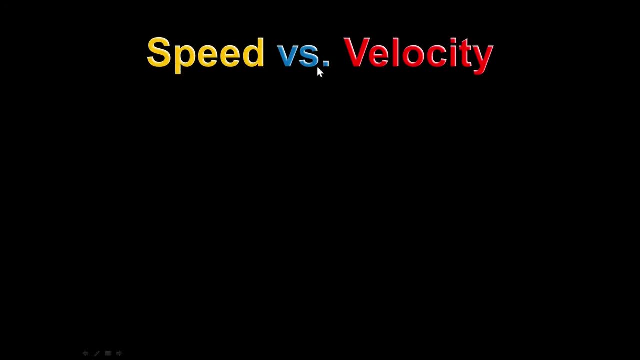 All right. Now we do make a distinction between speed and velocity. They're not the same thing. So velocity is defined as- And I'm going to tell you now that these three little lines here is different than two little lines. It's better than being equal. 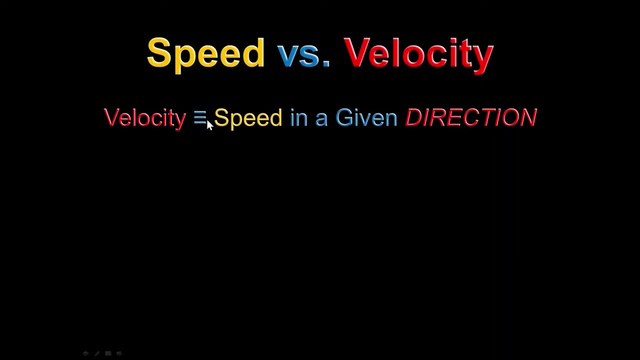 This is the very definition. So three little lines means the definition. So velocity is speed in a given direction. If you're going down the freeway and I ask you what is your speed, You could say 55 miles per hour. But if I ask you what is your velocity, 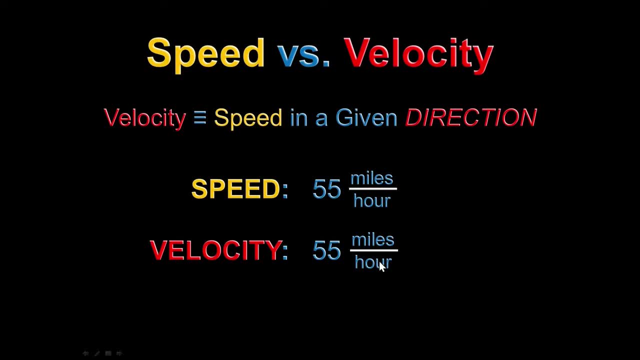 You shouldn't have the same answer because it really is a different question. So if I ask you what is your velocity, You could say 55 miles per hour, but you also have to state what direction you're going, because going 55 miles per hour to the east- 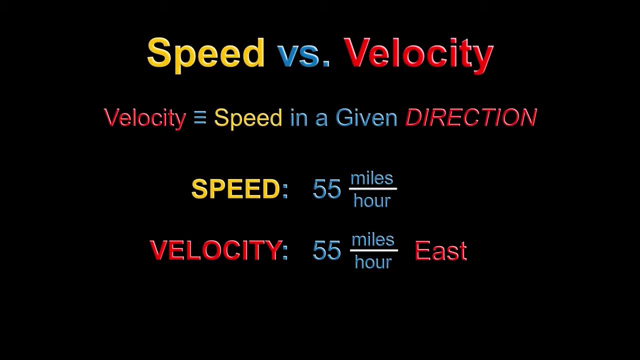 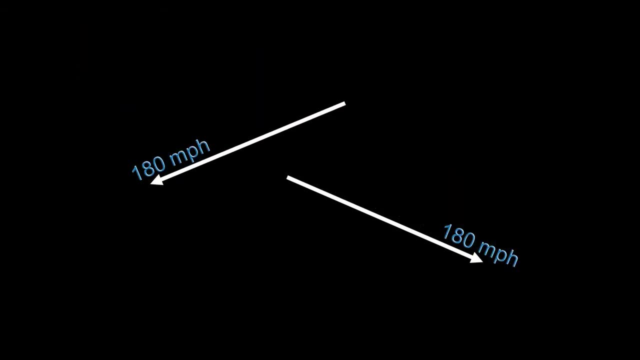 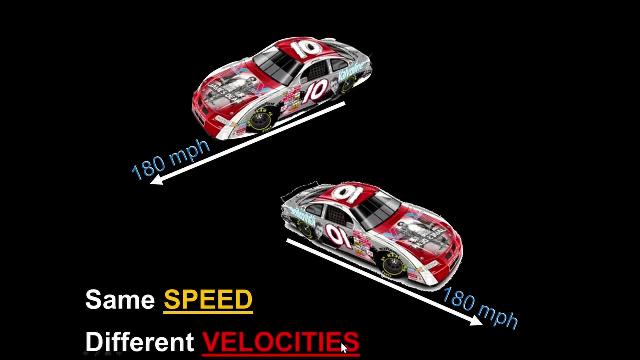 is different than going 55 miles per hour to the north. So if these two race cars are both going 180 miles per hour, those two race cars have the same speed, but they have different velocities In order to have the same velocity. 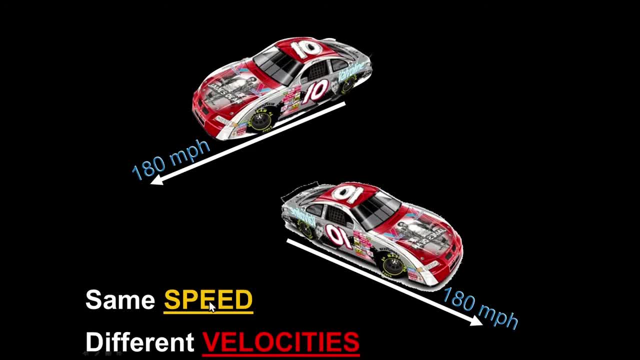 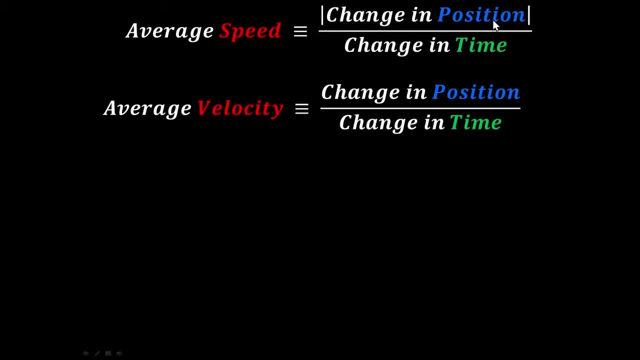 you need to have both the same speed and the same direction. So when we defined average speed as the absolute value of your change in position divided by a change in time, we're now going to define the average velocity as just your change in position divided by time. 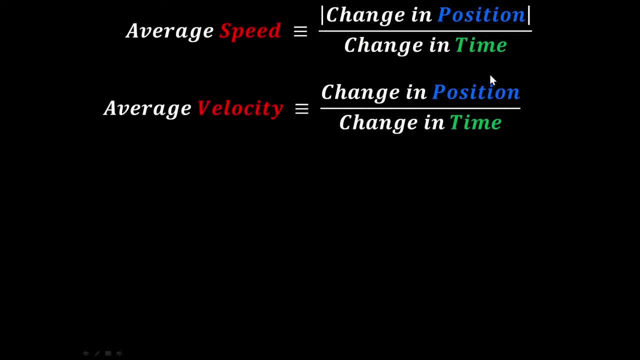 without the absolute value. So velocities can be negative. And if the velocity is negative it just means you are moving to the left. So we take our change in position divided by change in time, and this is what we come up with. We just say the velocity is final minus initial positions, divided by time. 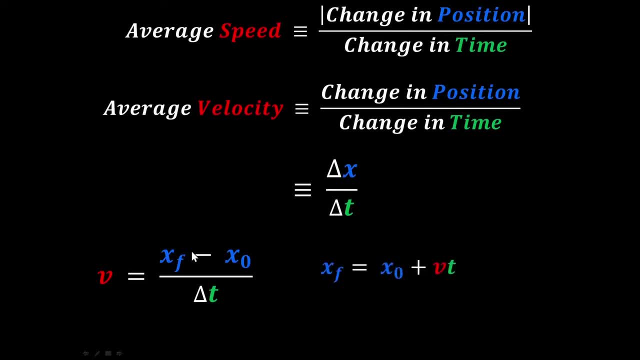 If we take that equation and solve it for the final position, we're going to multiply both sides by the change in time, or just the time, and then we're going to add the initial position to both sides. We come up with this equation here. 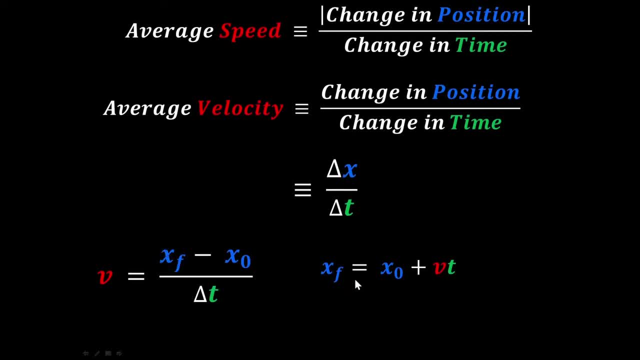 just rearranging that for the final position. What we can say is: this is the final position at this moment in time, So we can talk about this as being your instantaneous position at this instant, And this is how we typically see that equation And just the notation is just a little different. 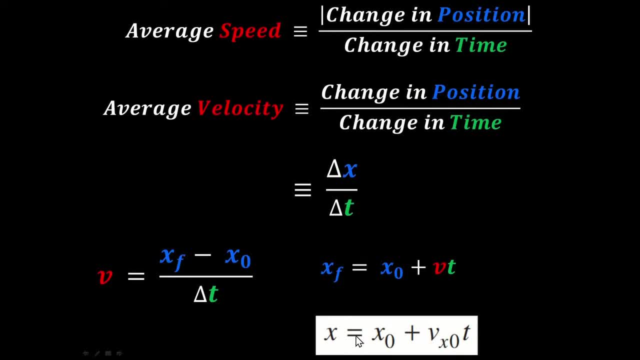 It just says what is our instantaneous position. it's going to equal what our initial position was plus how fast we were going for a length of time And this v sub x knot. this is meaning this is your initial velocity in the x direction. 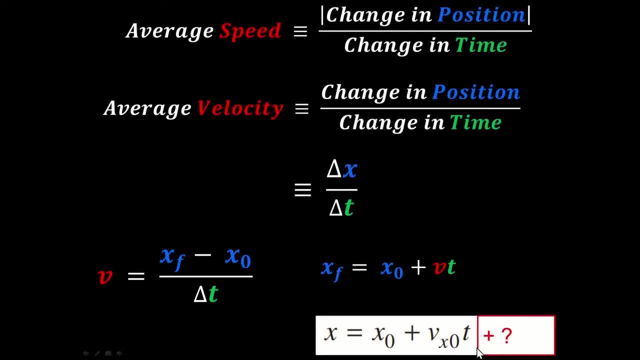 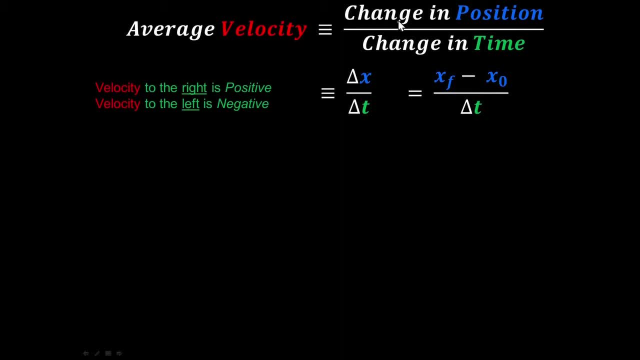 Alright, There is another piece that's going to be added onto this equation a little later, but we're not quite ready for that yet. So, because velocity can be negative, we're going to say that if you're moving to the right. 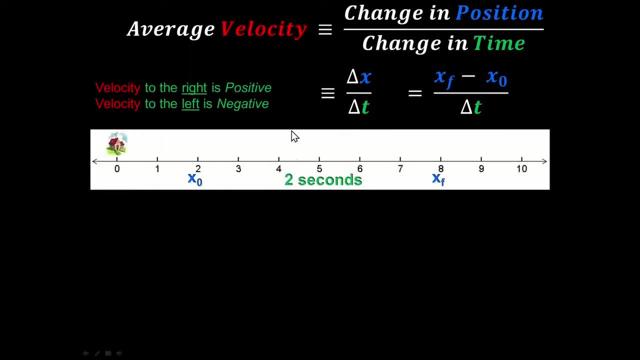 your velocity is positive And if you're moving to the left, your velocity is negative. So if this is a number line and this is home or the origin, if you go from 2 to 8, the way we find the change is it's always final minus initial. 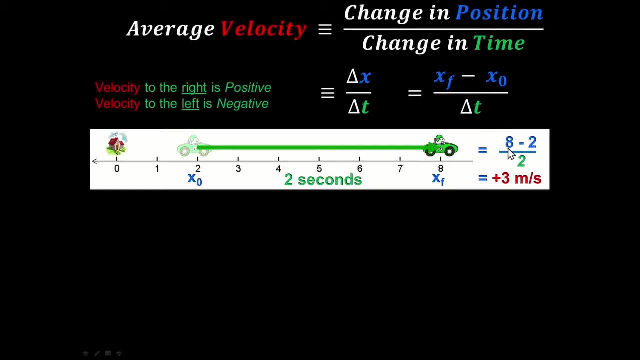 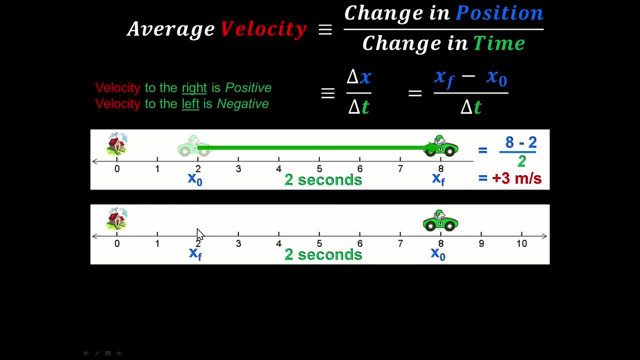 It's never initial minus final, Always final minus initial. So if I take my final position minus my initial position, I get 6 divided by 2, but I get a positive velocity, which means we were moving to the right If I go from 8 to 2,. 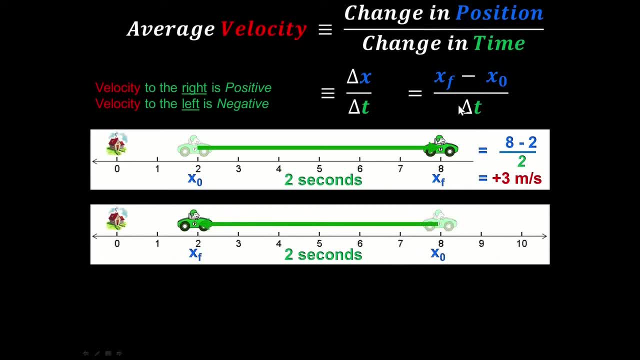 initial was 8, the final was 2, you stick with final minus initial. 2 minus 8 is minus 6, divide by 2, minus 3.. So this means that if you find your change in position and get a negative number, 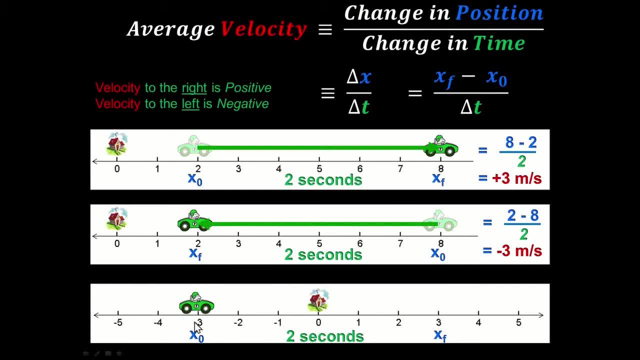 your velocity was to the left. And then if we go from, say, minus 3 to positive 3, you still do the final minus initial 3. minus a minus 3 is positive 6, divide by 2, it's positive 3.. 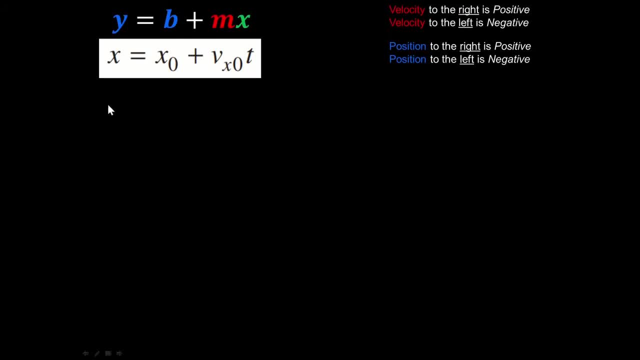 We were moving to the right. So there's this equation here and I want to compare that to the equation of a line. y equals mx plus b. Typically this term is first, but we can add in any order. So if we put time on the x-axis, 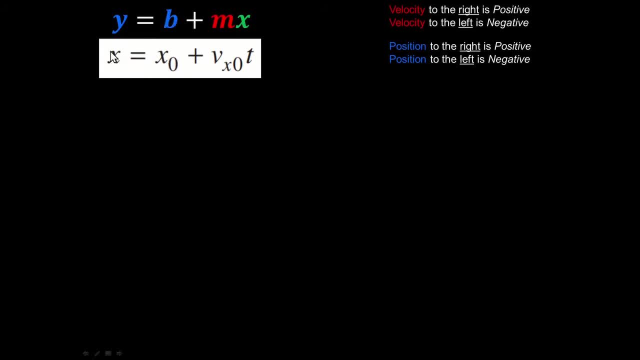 and the initial position as the intercept and the initial instantaneous x position on the y-axis. the slope of that is going to turn out to be the velocity. Now just don't be confused here. This x and this x are not the same x. 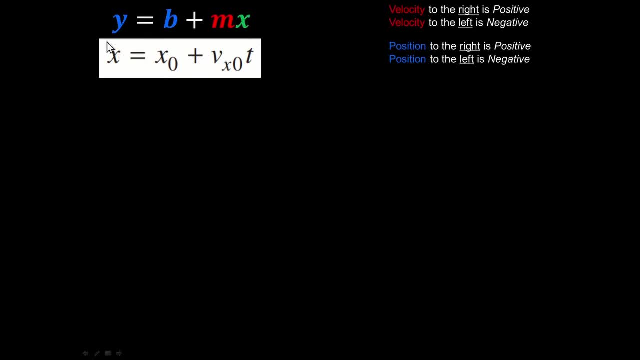 This is just what we graph on the x-axis and we're graphing time. This is what we graph on the y-axis and we're graphing position. So if I look at an example of that, let's say that I start out 100 meters from the origin. 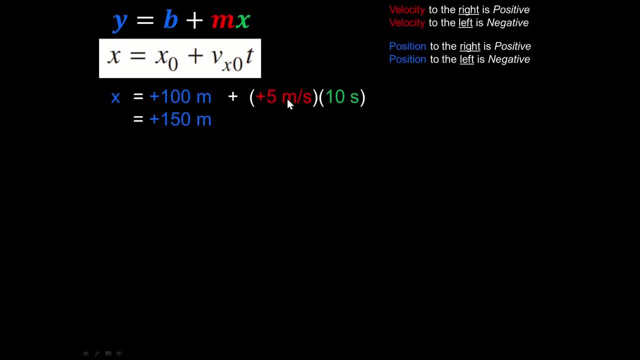 to the right of the origin, And then I begin moving at 5 meters per second for 10 seconds. That's 10 increases of 5 meters. You're going to change 5 meters every second, So you're going to travel 50 meters here. 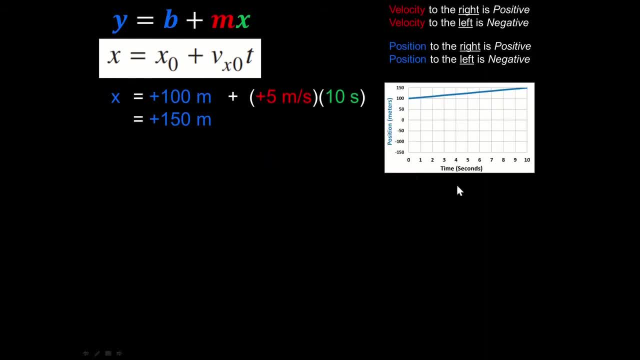 plus the 100 you've already traveled, That's 50 altogether. Graphing time on the x position. on the y, you can see we started out at 100, and over 10 seconds we moved over to 150.. And notice that is a positive slope. 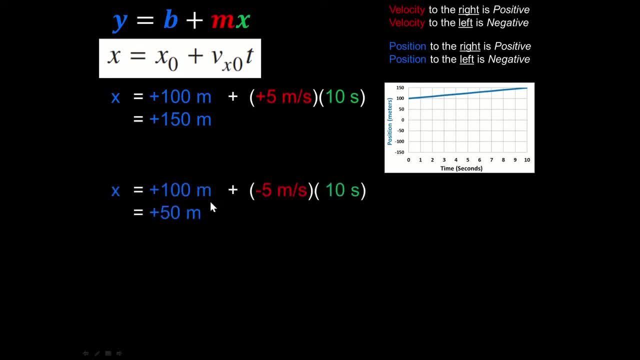 So the velocity here was positive If I start out at 100 meters from the wall, from some origin, and this time I have negative velocity, negative 5 meters per second, squared per second, and we do that for 10 seconds. 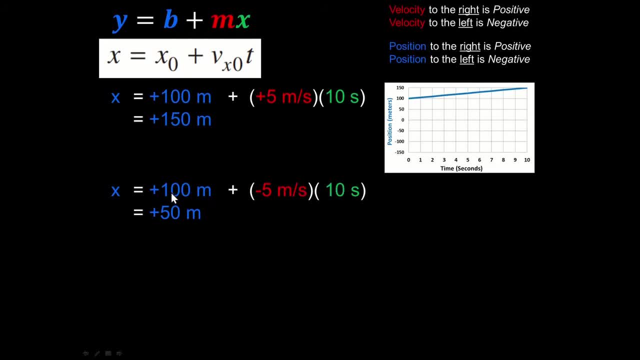 well, that means we're going to move to the left 50 meters, So we start out at 100, this time we have negative slope and by the time 10 seconds have gone by, we've gotten over here 50 meters from the origin. 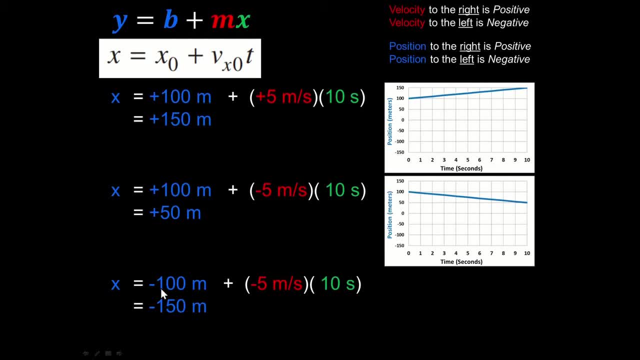 And if I start at negative 100 meters from the origin, that means I'm starting to the left and then now I'm going to have negative velocity. so we start out here at negative 100,. negative velocity means we're moving to the left. 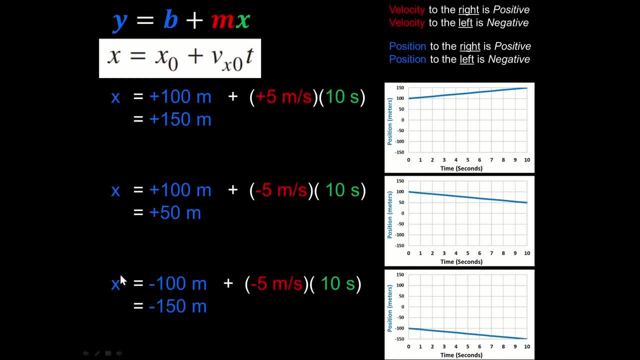 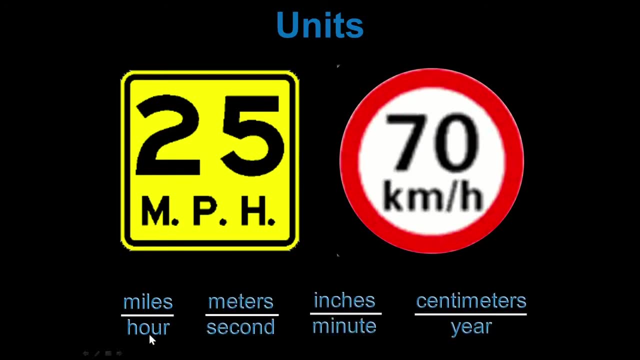 we're going to get even further to the left, So just be careful with your positives and negatives here. Units of velocity: any distance of time, any unit of distance divided by any unit of time would be appropriate units for velocity: Miles per hour, kilometers per hour. 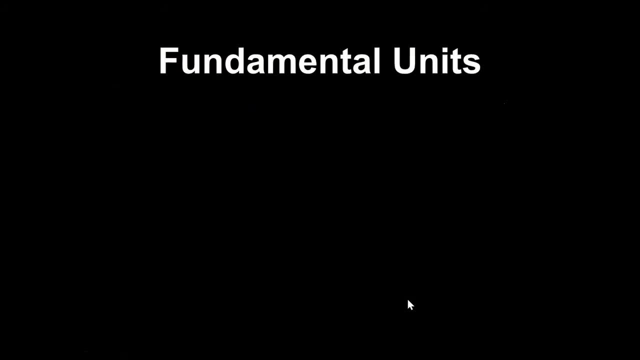 centimeters per year. any of those work. but in physics we're going to kind of limit ourselves to fundamental units. Fundamental means it can't be broken down any further. It's in its simplest form And we're going to use the MKS system. 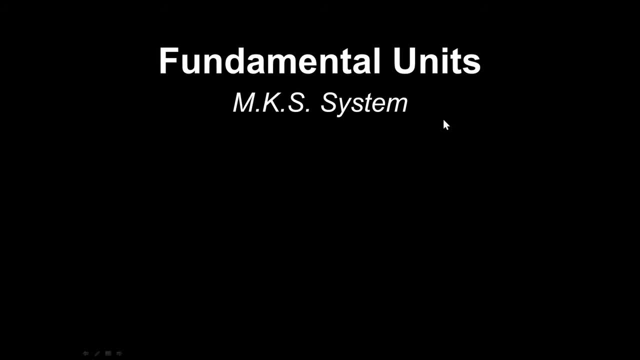 MKS system is a subset of the metric system, So we're going to M stands for meters, we're going to measure all distances in meters. We're going to measure all masses in kilograms and we're going to measure all times in seconds. 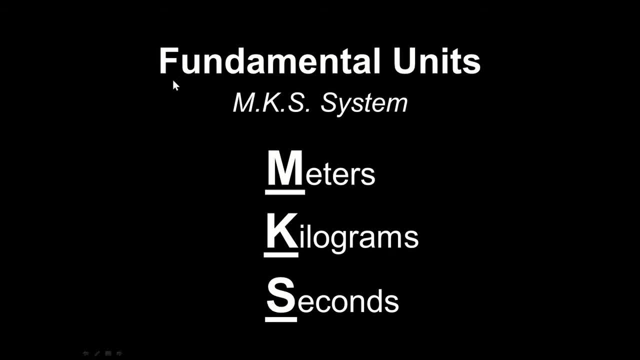 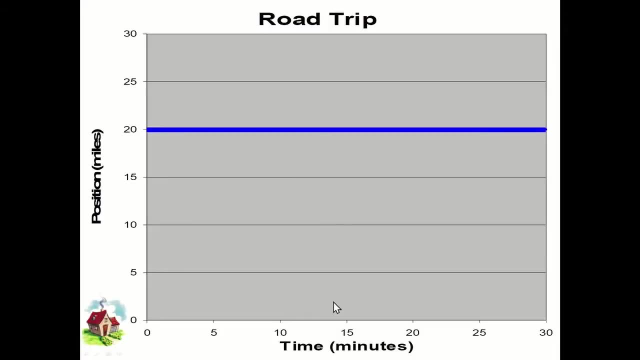 We're going to try to be consistent with that throughout this course. Now we can use other units just if we're familiar, but these are really the units we're going to focus in on. So if I have a graph of position and time, 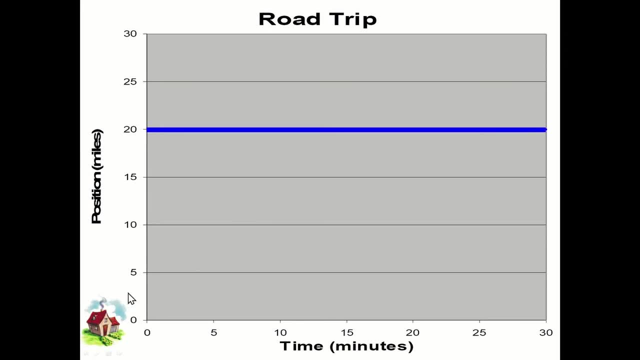 and I'm not using those units because I just want to do something a little more familiar. but is this object measured? Is it moving? And no, it's not, because as time progresses, you're staying 20 miles from home. You haven't changed your position. 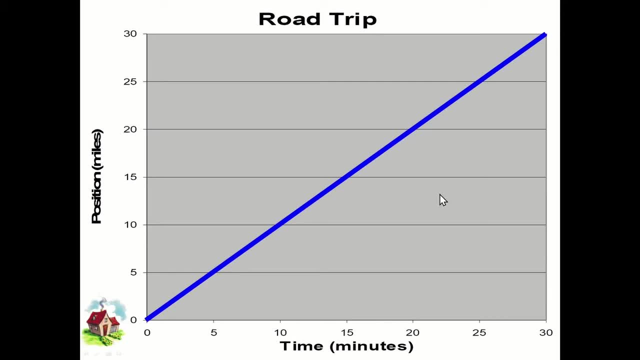 Is this graph moving? Represents something that's moving? And yes, it is Now, since average velocity was a change in position divided by a change in time, and we have to think about what slope means. It's rise over, run a change in the y coordinate. 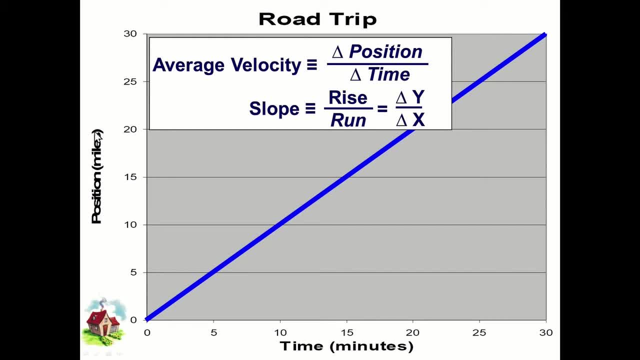 over a change in the x coordinate. So rise over run is a change in the position over a change in time. It looks like the slope of this graph would tell us the average velocity, This one here. let's say that we changed our position here. 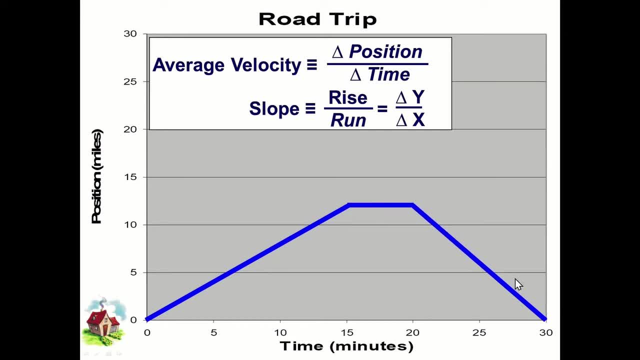 and through. here we are stopped and here we have negative slope, which means we're going backwards to the left. So where is the velocity the greatest? Students might be tempted to say that riding through here the velocity was the greatest. but we're not graphing velocity. 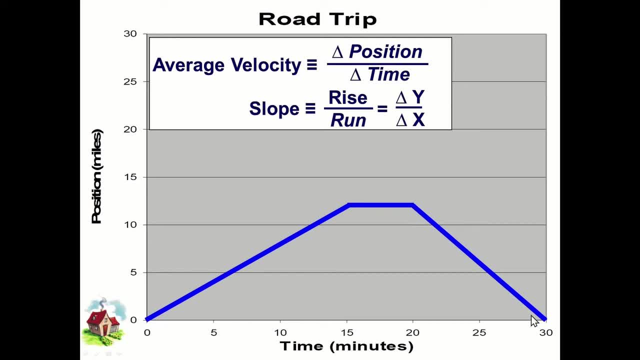 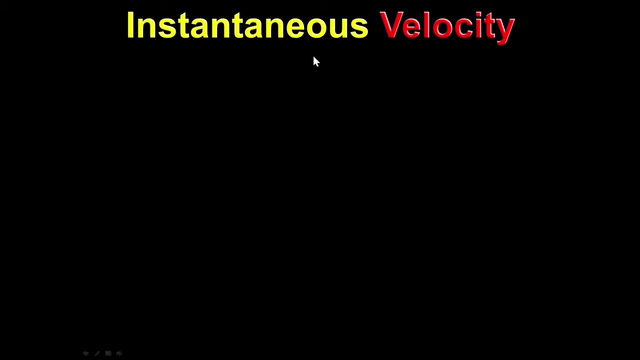 It's the slope that tells us the velocity, And because this slope is steeper, it means it has a greater velocity. All right, now let's talk about instantaneous velocity versus average velocity. Instantaneous velocity is just what is your velocity at that specific moment in time. 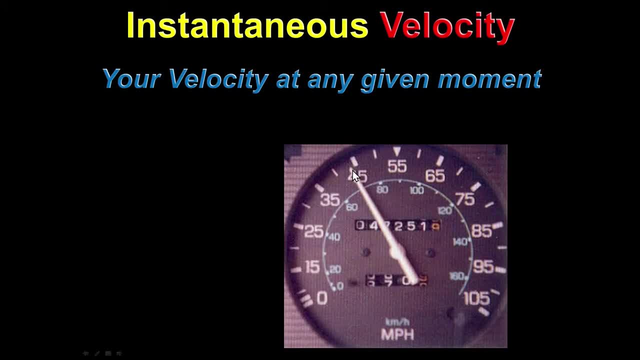 And you could look at a speedometer at some moment and see what your velocity is. Typically we measure that in miles per hour. If we did it in MKS it would be meters per second. A little bar over the velocity here indicates. 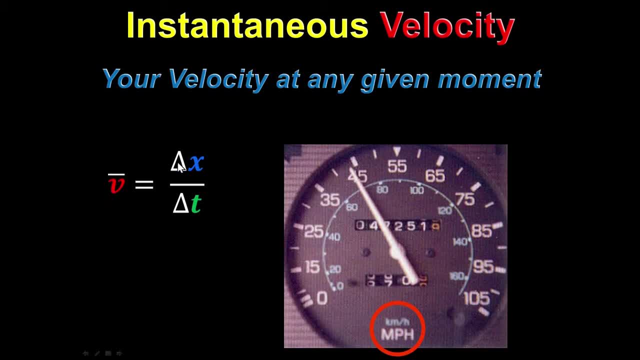 that that's an average velocity: a change in position over a change in time. Now what equation are we going to use to calculate instantaneous velocity? I want to just pause and understand, or remind you that this is an algebra course, not a calculus course. 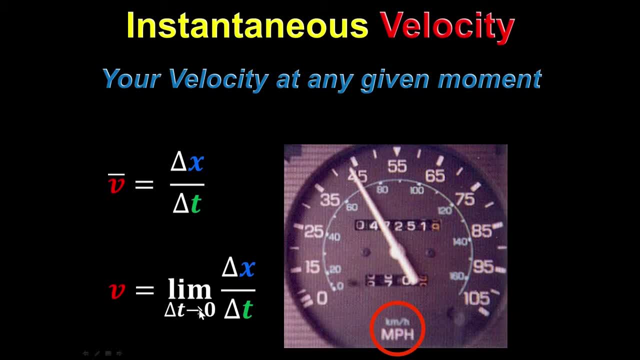 and this is kind of a calculus notation, But it just simply says what is the velocity going to be in what's called the limit, as delta t goes to zero. That means as the change in time gets closer and closer and closer to zero. 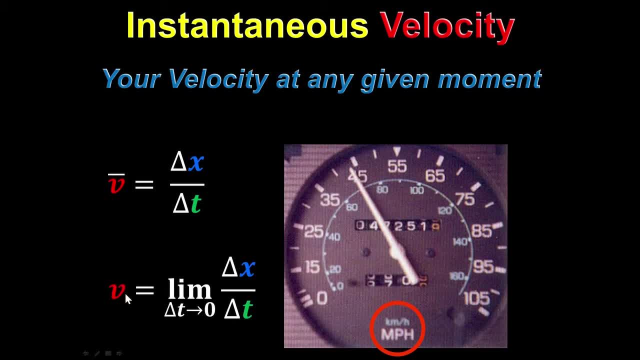 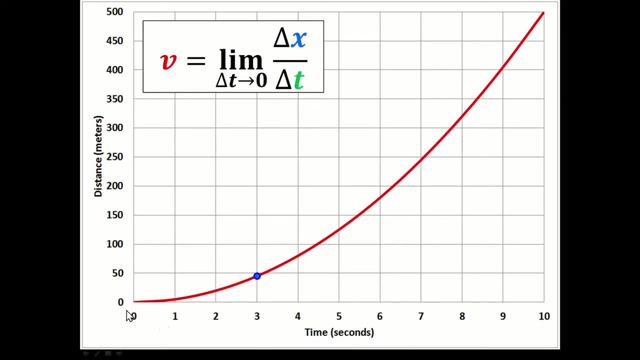 that would give us our instantaneous velocity. So don't be too frightened by that. We won't deal with that very much. But if we have position and time- and this time the graph curves- we could calculate our average velocity by finding the slope between two points. 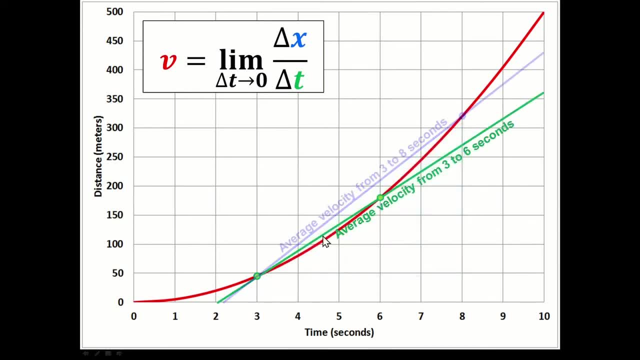 rise over run. If those two points are a little closer together, we could find the slope between those two points. Or if those points are even closer together, we can find the slope between those. But if these two points get closer and closer and closer and closer together, 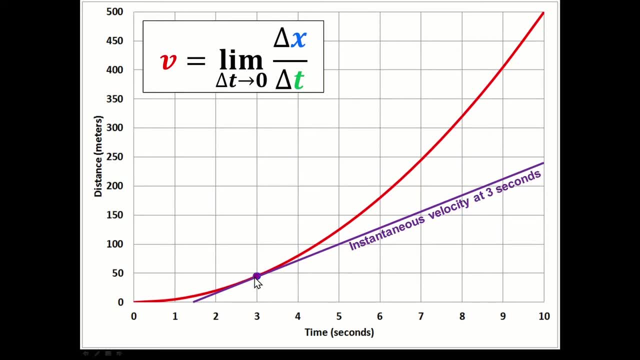 so close that they are actually one and the same point. we could still find the slope of that line by drawing the line tangent to that curve. So as the slope gets steeper and steeper and steeper and steeper, we can find the slope at that one point there. 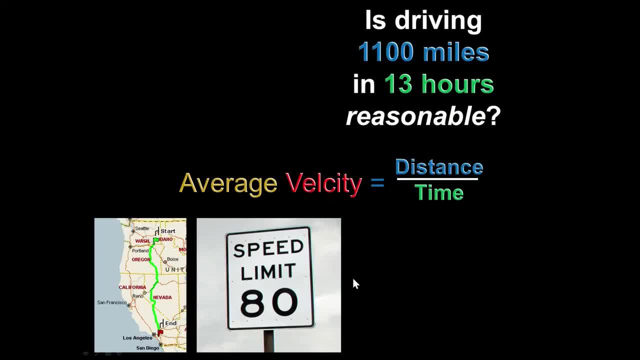 and that would be your instantaneous velocity at that moment. So let's see if we can identify the difference between instantaneous and average velocity. If you're doing a road trip and you drive 1,100 miles in 13 hours, is that reasonable? 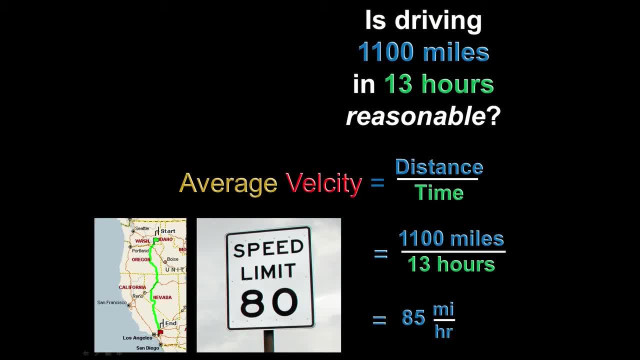 Well, 1,100 miles divided by 13 hours is about 85 miles per hour And you're going through Nevada and stuff and the speed limit there is probably 80 miles per hour, So going 5 miles an hour over. 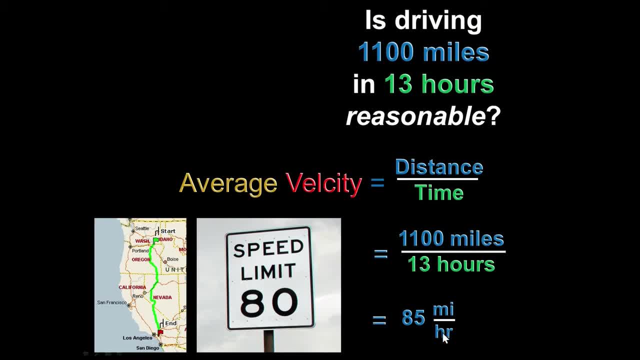 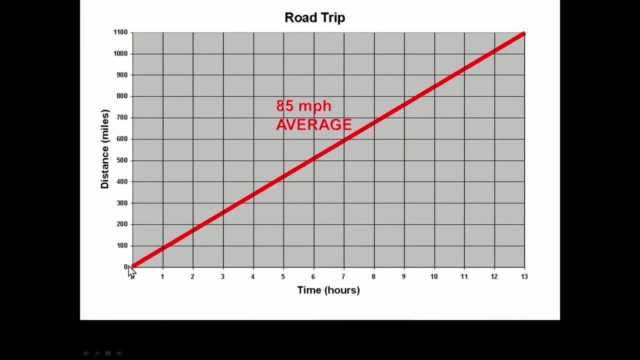 is that going to be an unrealistic thing? Well, if you say that's realistic, we have to be careful. That was my average velocity going from here, traveling 1,100 miles in 13 hours. But my average velocity is not the same thing as my instantaneous velocity. 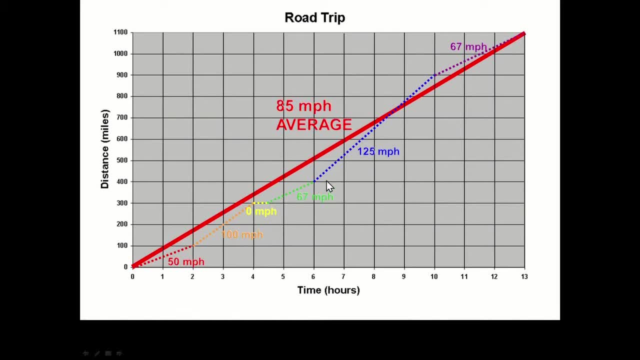 that you might be going here, then here and stop for a little while and then you have to go really, really fast to pick up that extra to increase your average. I see students make this mistake a lot- that typically students want to find. 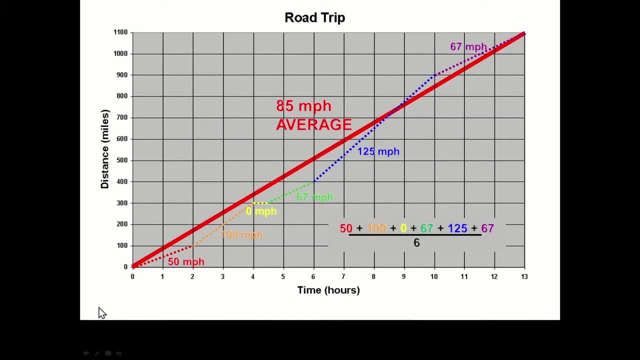 average, the same way they have always found average by just taking this, this, this: add up the six numbers and divide by six. It doesn't work here because if I add up those numbers and divide by six, I get 68 miles per hour. 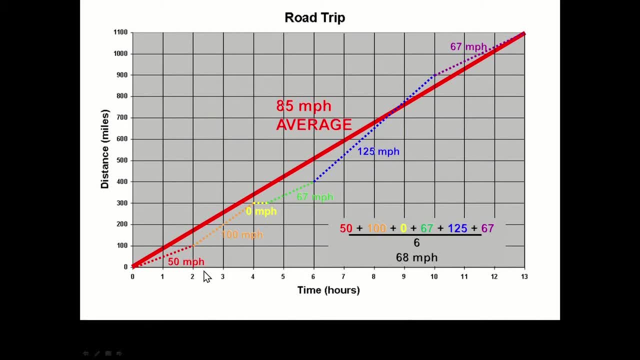 So just be careful You don't calculate average the same way you've always calculated average. It doesn't work. in this case. The reason is: here we're only going 67 miles per hour for a short period of time, and here we're going 125 miles per hour. 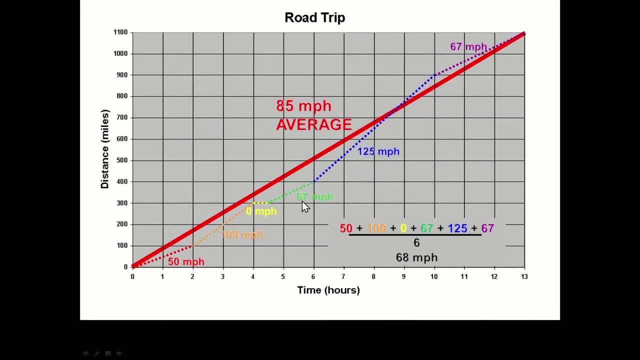 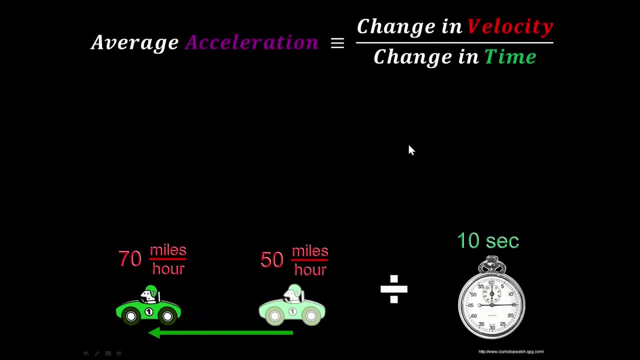 for a long period of time, So this doesn't carry the same weight as this because it was so much longer time. We have to stick with the definition: total distance divided by total time. Okay, so now that we've talked about change in position divided by time, 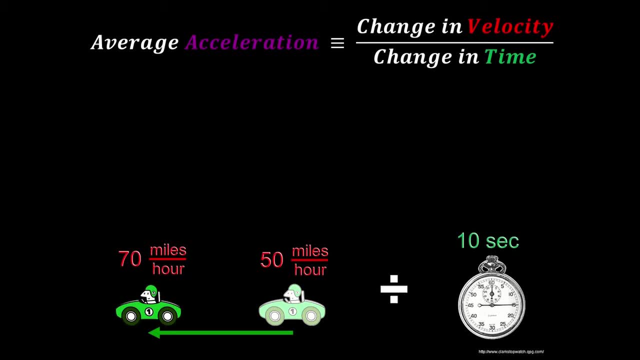 giving you the velocity, the average velocity. now let's talk about average acceleration. This is something that students really struggle with, so I want to just pause and make sure that we're talking about acceleration here. How you have defined acceleration in the past. 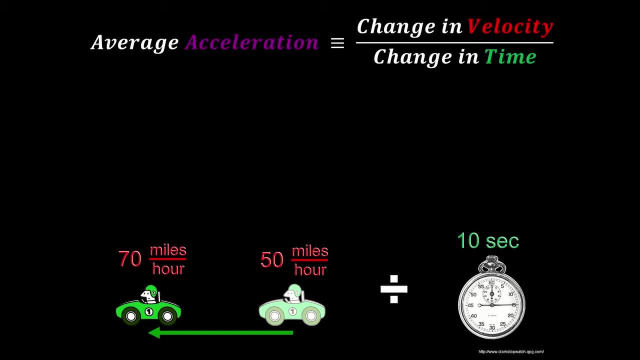 is probably not how we're going to define it from here on out. This is the definition. Three little lines is the definition. It's a change in velocity divided by a change in time. So if you're going 50 miles per hour, 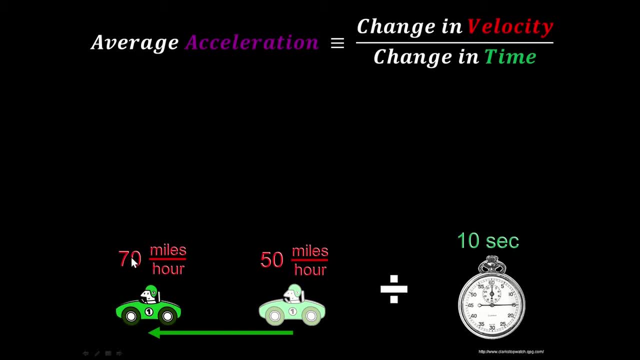 and then a little while later, you're going 70 miles per hour. you had a change in velocity divided by time, 10 seconds- and you could calculate your acceleration. So let's do that here. The final velocity was 70.. 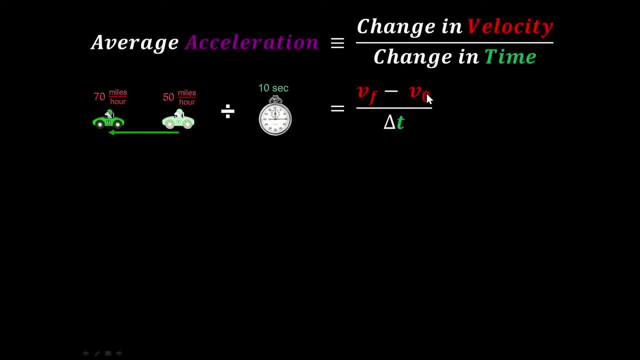 The initial velocity was 50. And we did that in 10 seconds of time And I think you could take those numbers there, plug them into the equation and come up with the number 2.. But what are the units going to be? 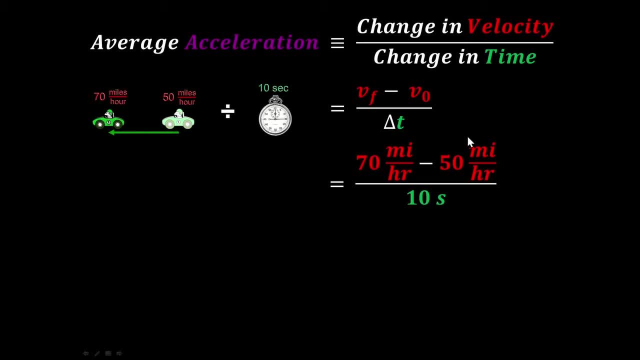 That's what's really important here, Because 70 minus 50 is 20.. Divide by 10 is 2.. But what are the units? So if I take 70 minus 50, I get 20 miles per hour, And I'm going to divide miles per hour by seconds. 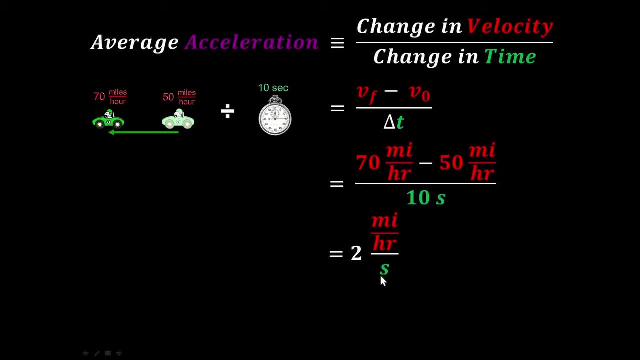 Miles per hour divided by seconds. If I put seconds over the number 1, I have a fraction over a fraction. Copy the denominator and flip it. Copy, dot, flip or copy dot, flop, We get this. So this is 2 miles per hour seconds. 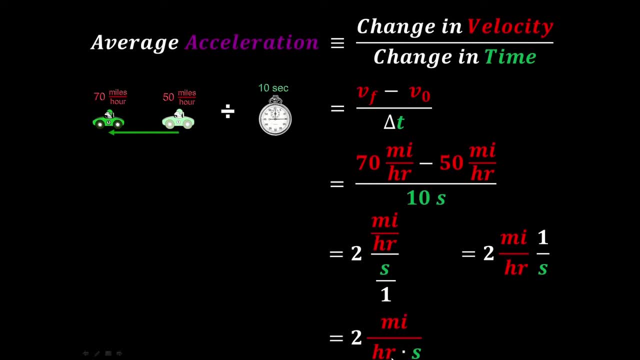 Which may not convey much information. as we initially start with this, Maybe it's clearer if we talk about miles per hour per second. Miles per hour per second. What that means is every second that goes by, we're going to change our velocity by 2 miles per hour. 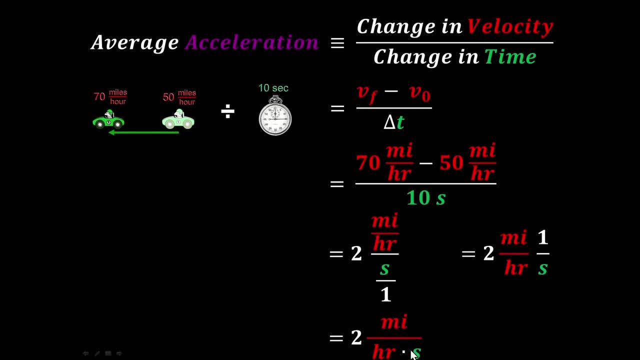 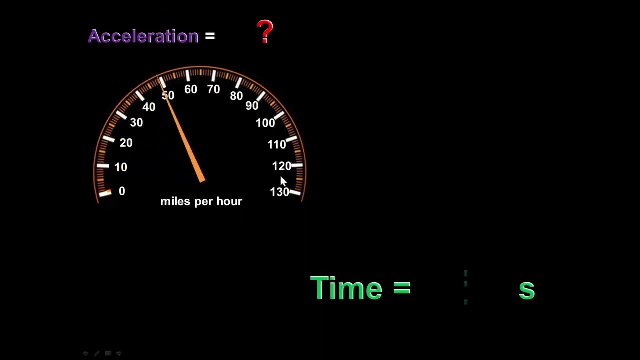 But algebraically it's the same thing as 2 miles per hour, seconds, Alright. So let's see if we can estimate the acceleration of this car And see if you can estimate it before the time stops, When we had a total change in velocity. 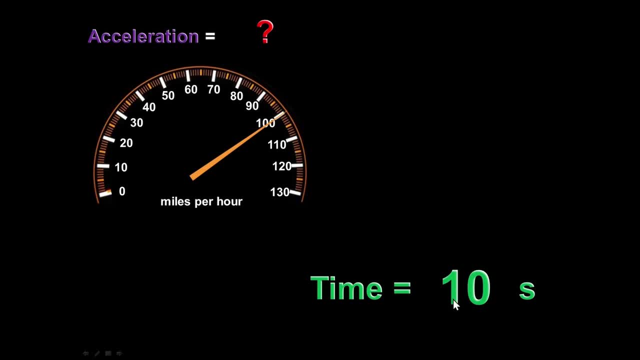 of 100 miles per hour in 10 seconds. the acceleration is 10 miles per hour per second. Every second we change our velocity by 10 miles per hour. Let's see if we can do this one. now We're going to start the time. 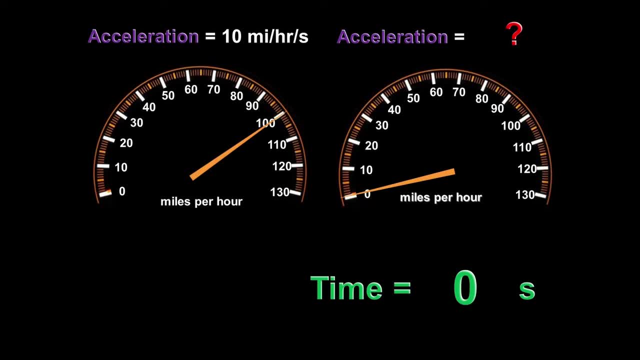 and I want you to see if you can estimate your acceleration before the time stops. Okay, so hopefully you're starting. You can kind of estimate And that is going to be a change of 50 miles per hour in 10 seconds, And that's 5 miles per hour per second. 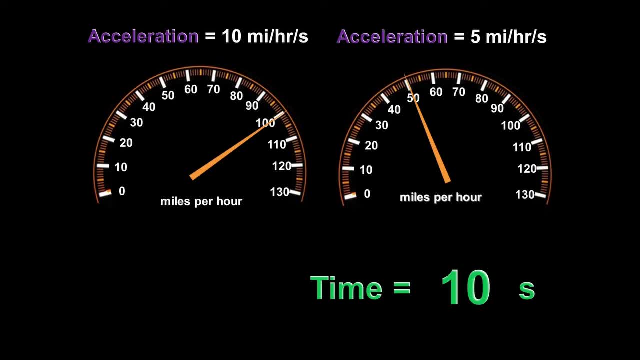 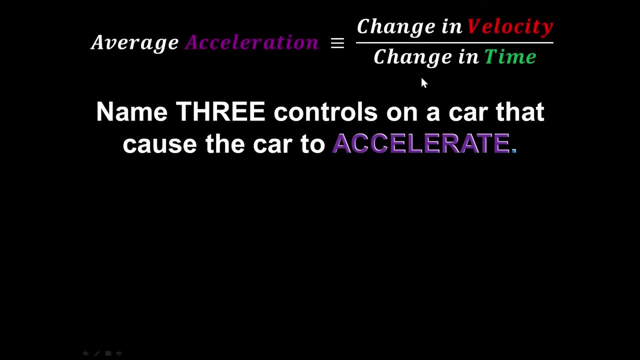 So maybe if you could pause and think. when you're stopped at a stoplight light turns green, you're not in a hurry. at what rate do you typically accelerate? Think about the next time you drive. Alright, if this is the definition. 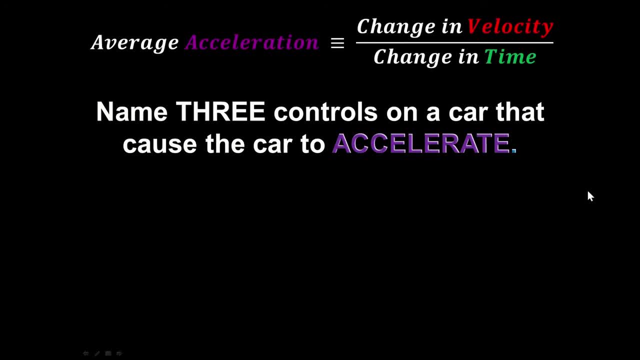 of acceleration. what are three controls on the car that cause the car to accelerate? Well, one would be the gas or the accelerator. The brake would be another control on the car that causes the car to accelerate. When you hit the brake, you are accelerating. 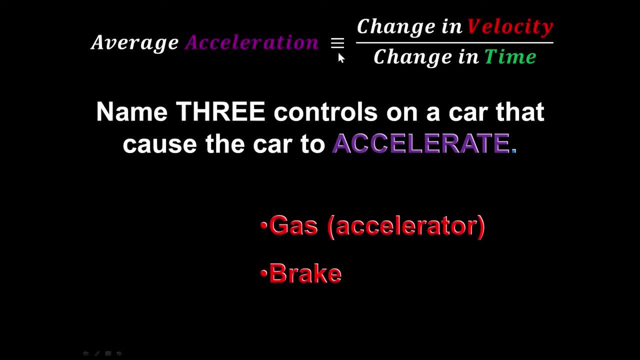 Because accelerating does not mean going faster. Its definition is a change in velocity over a change in time. So when you hit the brake it causes you to change your velocity, It causes you to slow down. but that is acceleration. And the third control is the steering wheel. 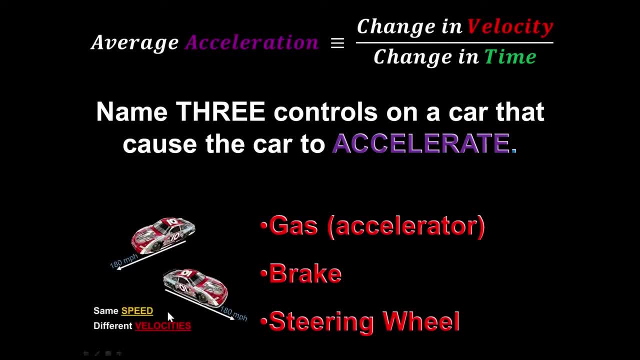 Now, how does the steering wheel cause you to accelerate? Well, remember that these two cars have the same speed, but they have different velocities. If this car goes 100 miles per hour that way, and then a little 180 miles per hour that way, 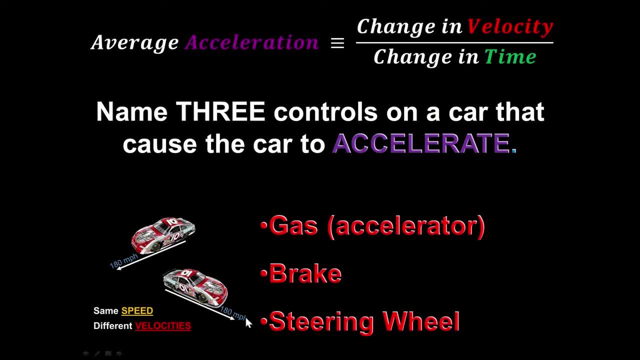 and then a little while later it's going 180 miles per hour. that way it has a different velocity, So it has changed its velocity. Turning is an example of accelerating, because changing your direction is changing your velocity over time. So if you're in this car going 70 miles per hour, 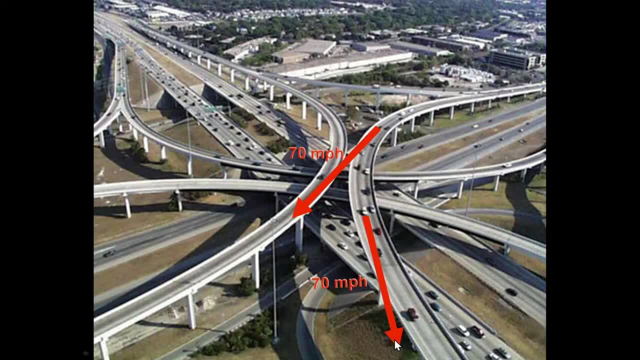 and then a little while later, you're now going 70 miles per hour. you've accelerated because you have changed your velocity. This velocity is different than this velocity, even though this speed is the same as this speed. So when you go around a turn like this: 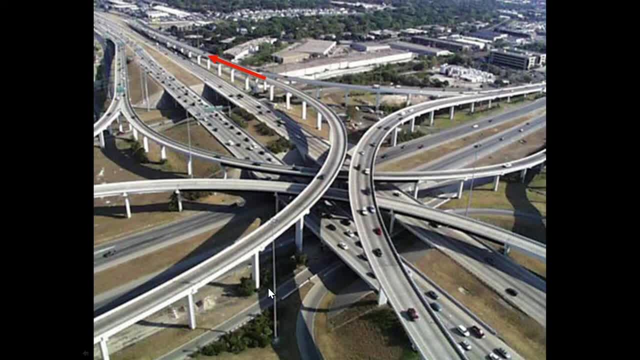 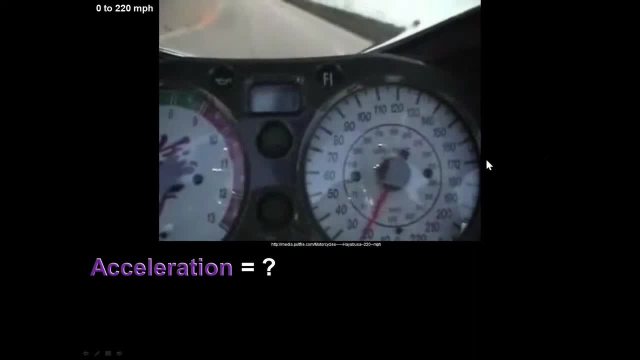 you are accelerating the entire time. you're changing your velocity. So here's a motorcycle and we're going to start the time. we're going to keep track of the speedometer here and you can see it's really changing your velocity There. you're changing your velocity a lot. 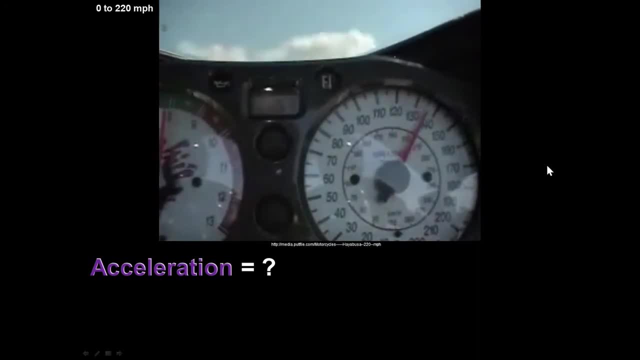 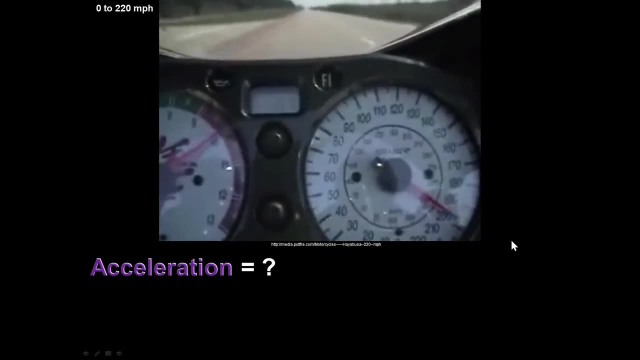 You're seeing Sky doing wheelie, And then now we're continuing to accelerate. we're still going faster and faster and faster and faster, all the way up to 220 miles per hour. A little disclaimer: don't try this, please. But if it took 25 seconds to go from 0 miles per hour, 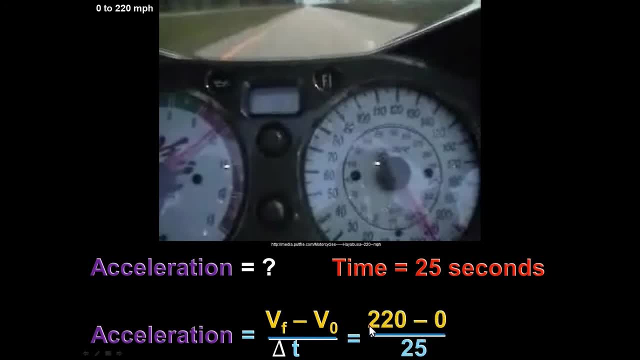 to 220 miles per hour. that's a change of 220 miles per hour in 25 seconds. You divide those out and you get about 8.8 miles per hour. That's miles per hour per second or just miles per hour seconds. 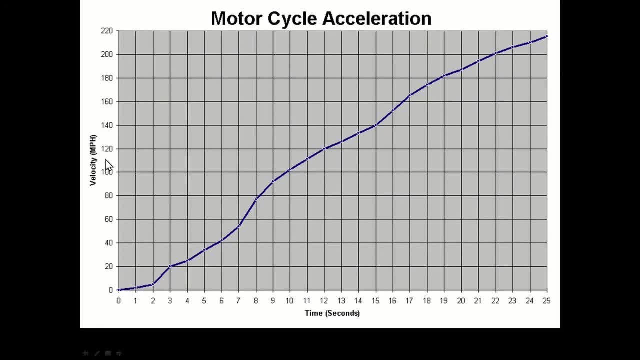 And if you look at the velocity, this is graphing velocity and time. Previously we looked at position and time. The acceleration is a change in velocity over time. but remember slope is rise over run or a change in the y-coordinate over a change in the x-coordinate. 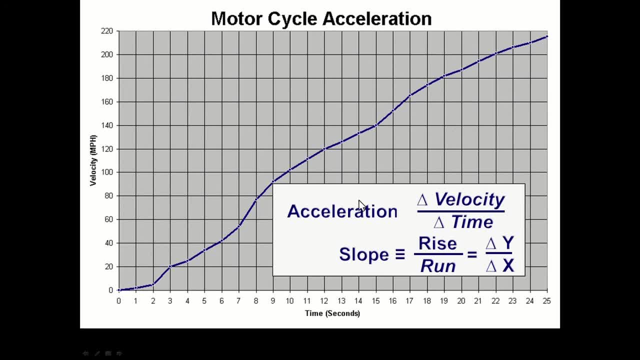 So a change in velocity over a change in time. It looks like the slope of this line tells us acceleration And that would be the average. But you can see that in through here the slope was a lot steeper and out through here the slope was less. 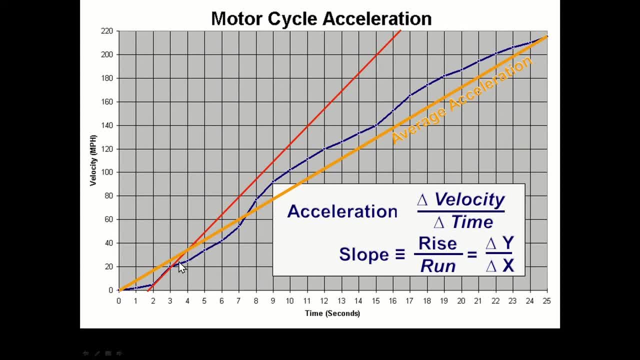 So if we choose two points that are really close to each other, it would tell us our instantaneous acceleration, And this is our average over just one second, and even between seven and eight seconds, the acceleration was just a little bit steeper, a little bit greater. 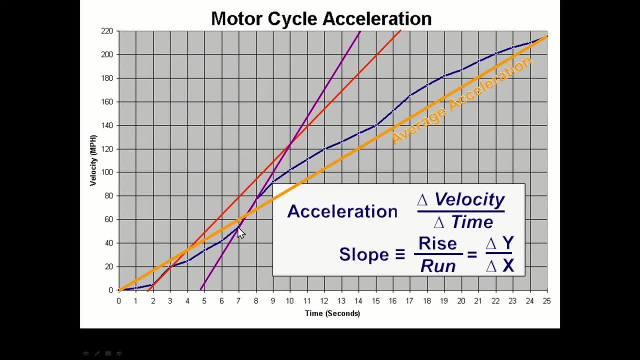 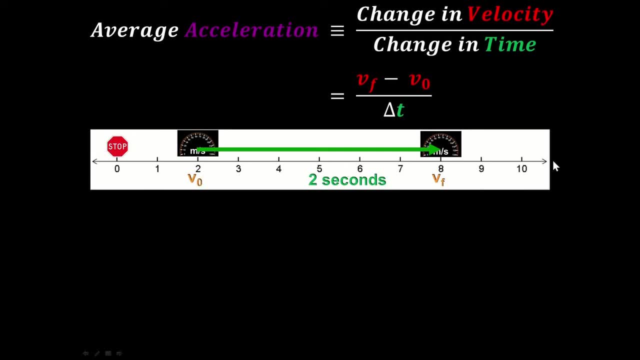 But if I were to find the slope at just one second, that would be our instantaneous Alright. we have this graph here. This time our number line is not position, it's velocity. So we started at two meters per second and we went to eight meters per second. 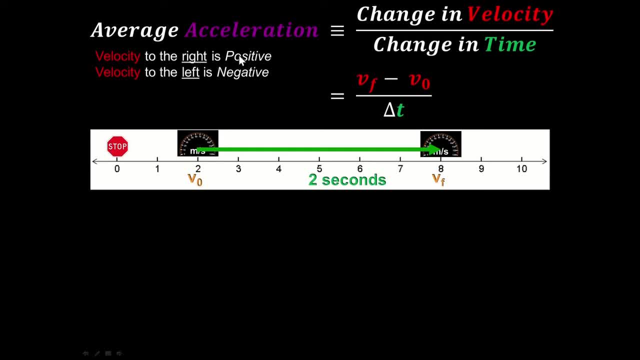 We're going to do the same thing where velocity to the right is zero, to the left is positive and velocity to the left is negative. Same thing with acceleration: To the right is positive and to the left is negative. So if I take final minus the initial, 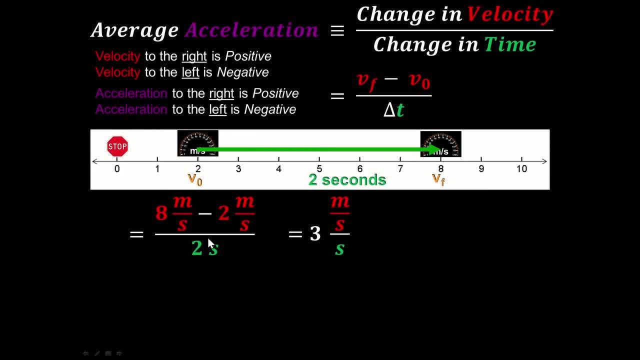 divided by the change in time, I'm going to get six. divided by two, I'm going to get three meters per second, per second, And if we put this over one, we have a fraction over a fraction and we get three meters per second. per second. 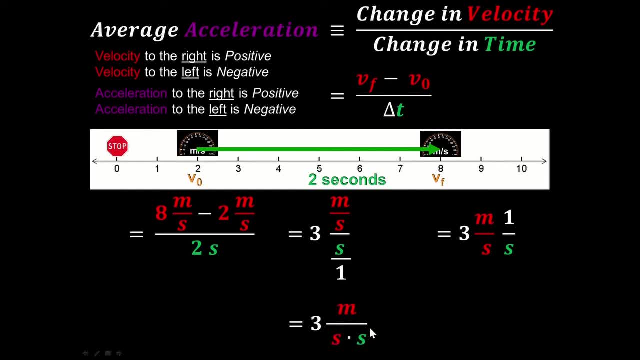 which means every second our velocity changes by three meters per second. Algebraically that's the same thing: Seconds times seconds is seconds squared. So this is the first time we're introducing this unit: meters per second squared. Don't be confused. 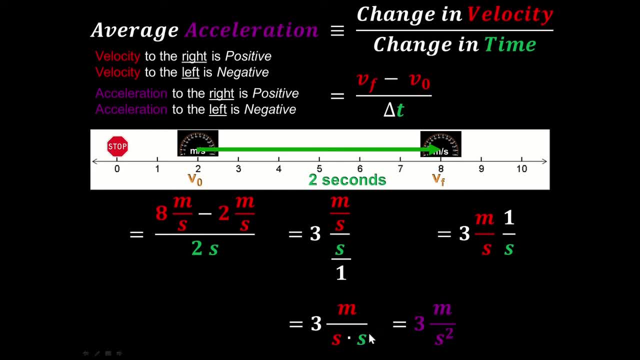 it's just, there's a seconds in there for the change in time and there's a seconds in there for the change in velocity, So we can find our acceleration. Our acceleration was positive here, because this thing was accelerating to the right, The velocity was to the right. 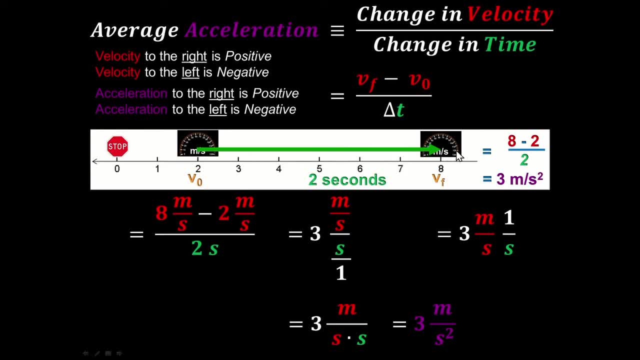 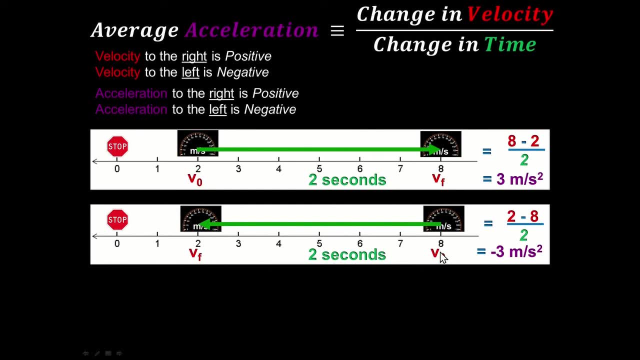 but the acceleration was also to the right. Now, let's say we start out at eight meters per second. That's a positive velocity. The thing is moving to the right and it's moving to the left. The thing is moving to the right. 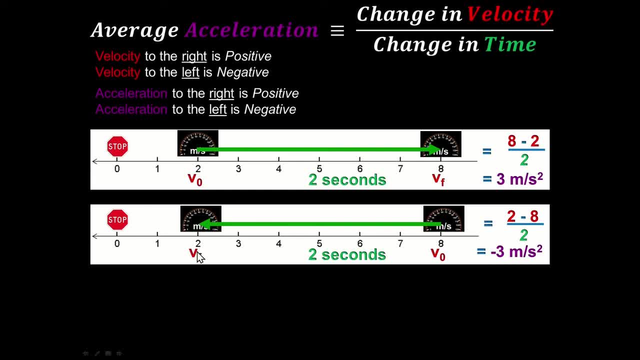 And then we go to two meters per second. It's still moving to the right. The velocity was to the right, But if I take final minus initial, I get a negative acceleration. So the velocity was to the right, but the acceleration was back to the left. 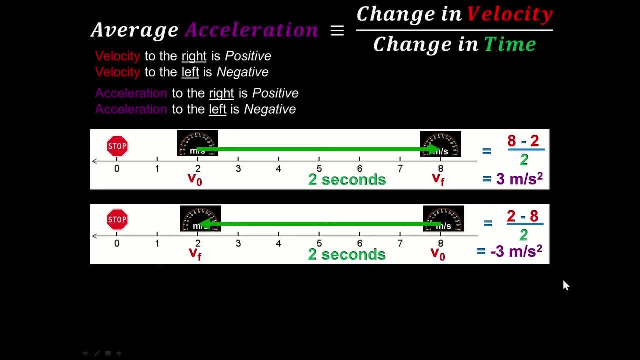 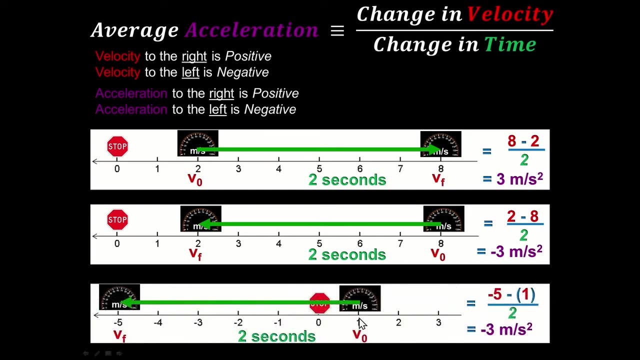 And any time velocity and acceleration are in opposite directions, you're slowing down. Any time the velocity and the acceleration are in the same direction, you're speeding up. So if we go from one meter per second, that means we're going to the right at one meter per second. 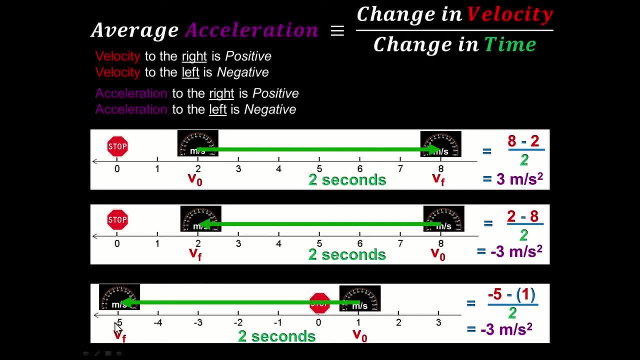 And then now we're going to the left at negative five meters per second. We're slowing down, slowing down, slowing down. We've stopped for a moment, And then now we're going faster and faster and faster and faster, but off to the left. 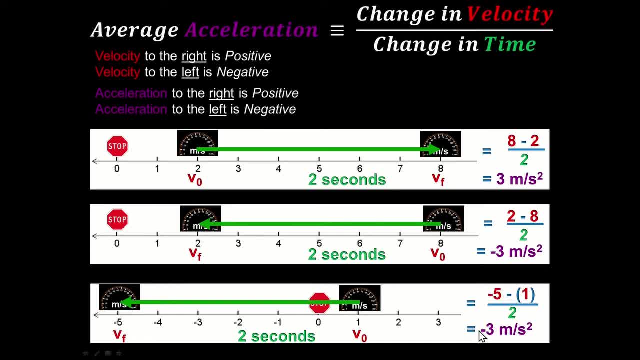 We're consistent with final minus initial. We get a negative acceleration, But the velocity is to the left, which is negative, and the acceleration was also negative. You're going faster and faster and faster and faster to the left. Sometimes we see negative acceleration. 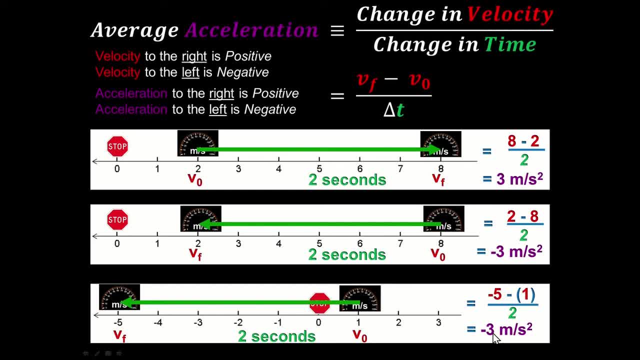 called deceleration. But the only thing that's different there is that we are assuming the velocity is in the positive direction. So if we assume the velocity is in the positive direction and we have negative acceleration, then that's going to be deceleration. 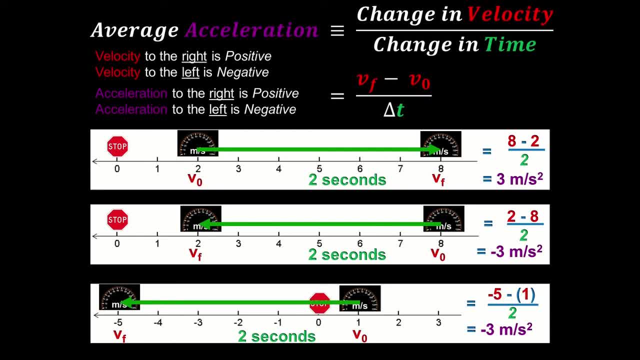 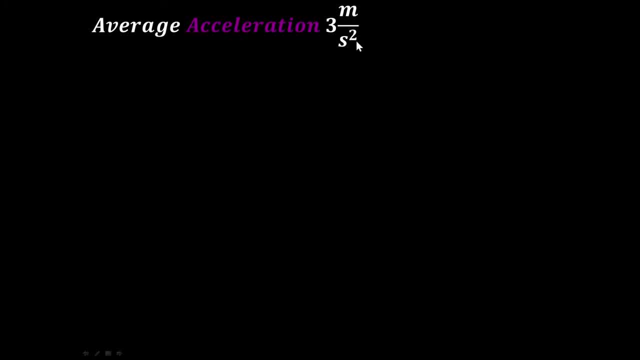 because the velocity and the acceleration are in opposite directions. So if we have an average acceleration of three meters per second, squared, what that means is again is that every second the velocity changes, whether it be getting greater or getting smaller, but the velocity changes by three meters per second. 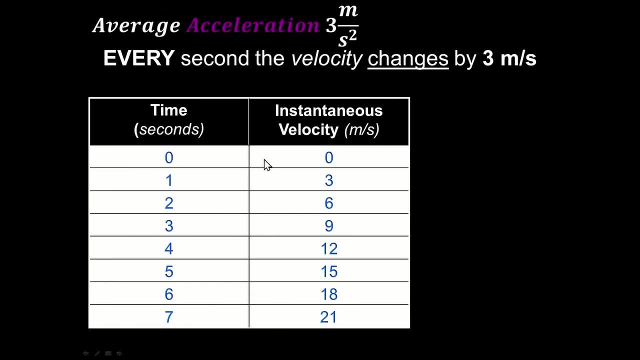 So if I had a table here at time zero, we're stopped at one second three, but we can see that every second that goes by, our velocity changes by three meters per second. Now if we maintained that acceleration for 30 seconds, 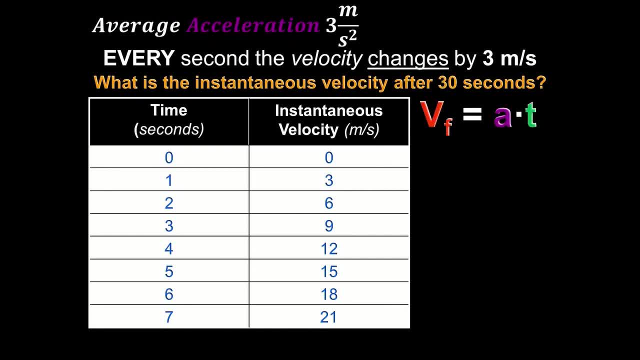 how fast would we finally be going? Well, hopefully you can see that it is going to be just acceleration times time, because if we do this acceleration for no seconds, we'll be stopped. If we do that acceleration for one second there, if we have done it for two seconds, 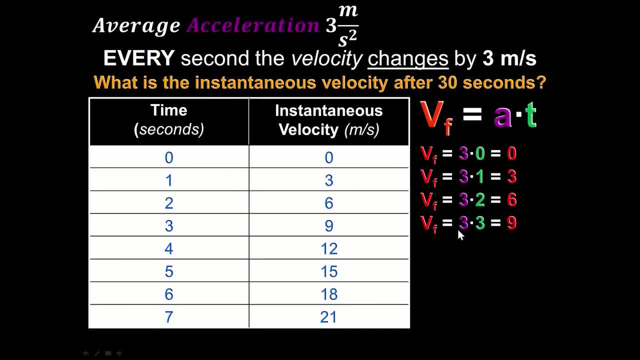 that's two increases of three, Three increases of three, and it looks like just taking acceleration times time would give us our velocity, our instantaneous velocity. So the final velocity is acceleration times time. Now, this is an equation that you can see. 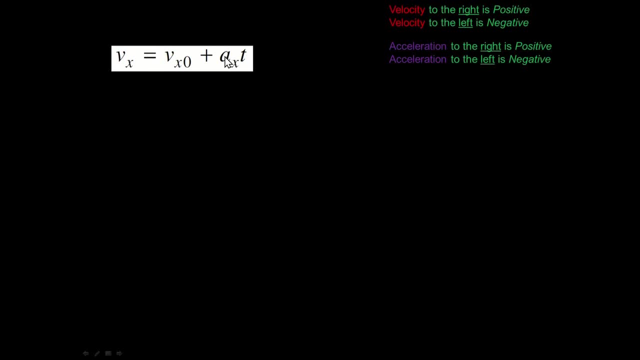 This is acceleration times time. It just is saying the acceleration in the x direction multiplied by time it'd be how fast you're going in the x direction. But if I add to that what we were already traveling at the initial velocity in the x direction, 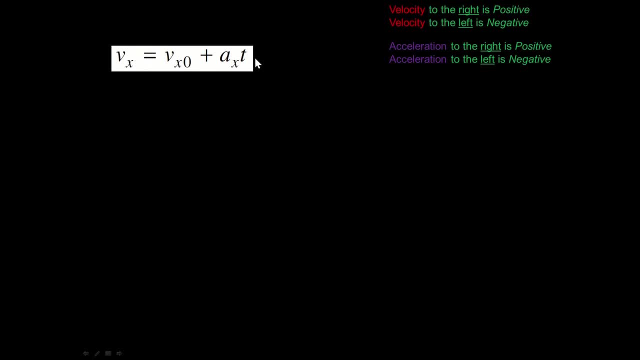 that would give us what our instantaneous velocity is at that moment. Comparing that again to the linear equation, y equals mx plus b. if I graph time on the x axis, velocity on the y axis, the slope is going to be our acceleration. 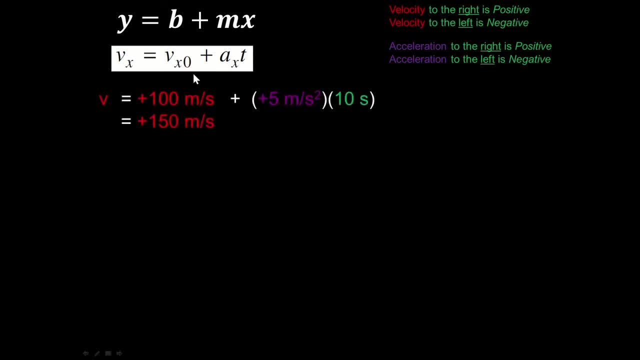 and our intercept is going to be our initial velocity. So if I start out at time zero, our initial velocity is 100 meters per second positively, so it's to the right, and then I begin accelerating at 5 meters per second, every second. 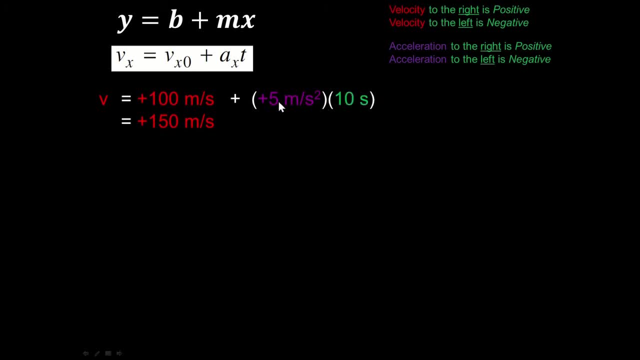 for 10 seconds. that is 10 changes of 5, that's going to get us up to 150 meters per second. So if we graph velocity and time, we start out at 100, we have positive slope, positive acceleration. 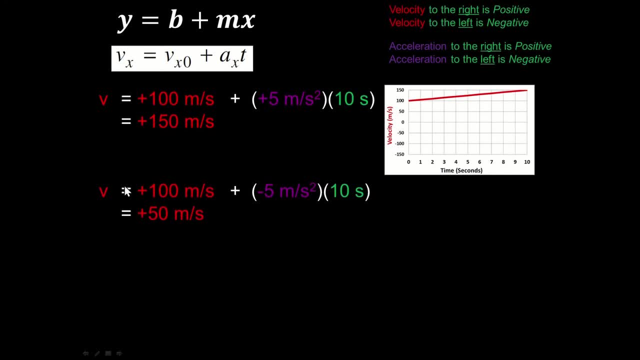 we got going even faster: 150.. If I started out at positive 100 meters per second, we're traveling to the right at 100 meters per second and I change my velocity by this much every second for 10 seconds. that's going to be slowing down. 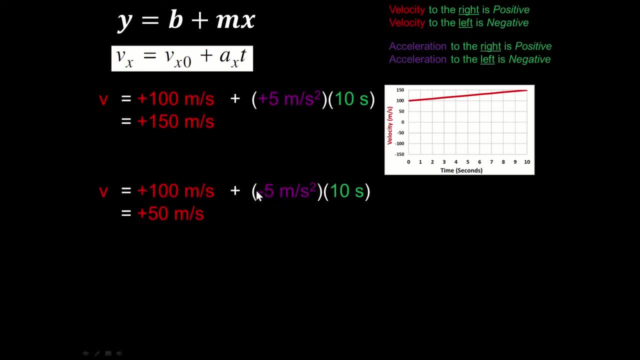 because I was going to the right and the acceleration was to the left. we're going to be slowing down, So this time our slope is negative. we start at 100, and over 10 seconds we got to 50 meters per second. 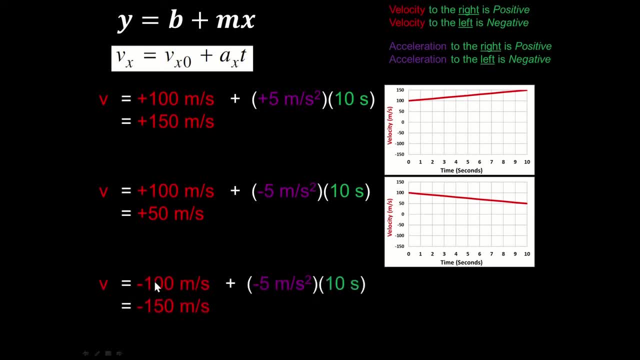 And then let's say that this time we were moving to the left at 100 meters per second- negative. and then we begin to accelerate to the left at 5 meters per second, every second. Do that for 10 seconds. we'll be going even faster to the left. 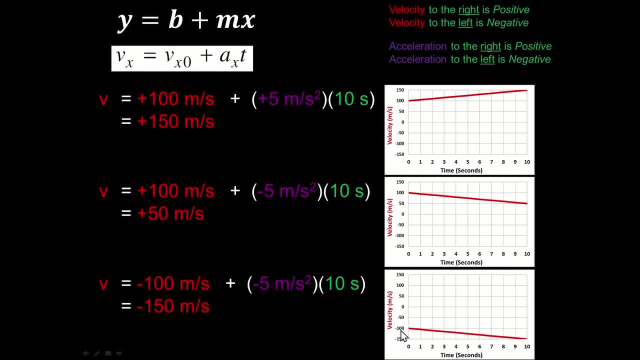 So it's like starting down here at negative 100, and going with negative slope it gets us even further down on our velocity. So this just reiterates that if the velocity and the acceleration are in the same direction, it's going faster.